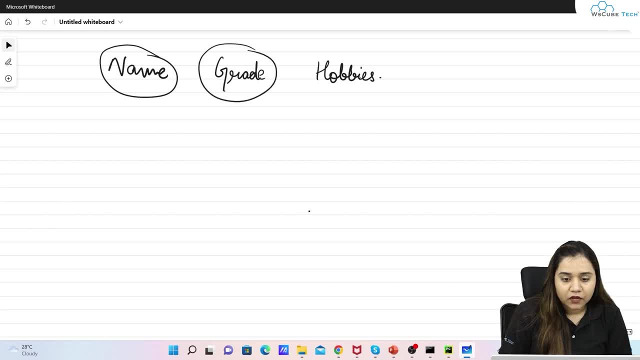 three parameters: The name will become the index, the grade will become the columns and the hobbies will become the data inside it. Suppose if we have, let's say, John, Peter, David and Lisa. Similarly, in the grade, we have third, fourth, sixth and eighth, and the hobbies we have dancing, singing, art and music. 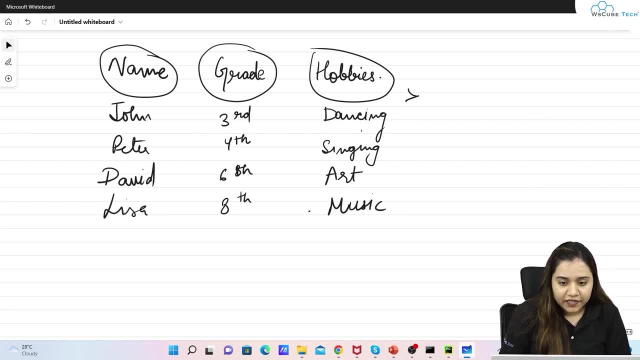 Okay, so now what new output we will get after pivoting. We will get the name. The names will remain like John, because it will become Rose, So Peter, David and Lisa. But now the grades will become the columns, So we will have third, fourth, sixth and eighth and the. 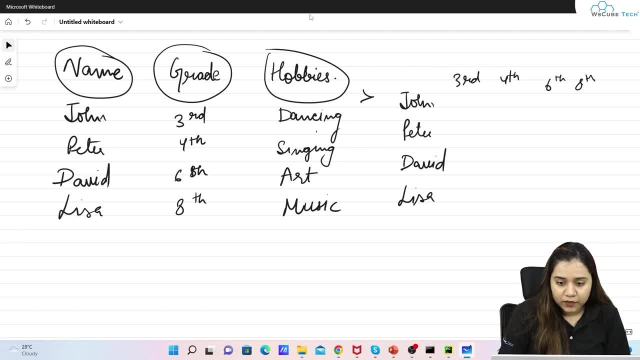 data over here would be. So John third and dancing. So hobbies would be over here. Here we will be having dancing. Here we have Peter, fourth, singing. So Peter over here. fourth over here. So here we will have singing. Here we will have it's not singing, but singing. Here we will have art and 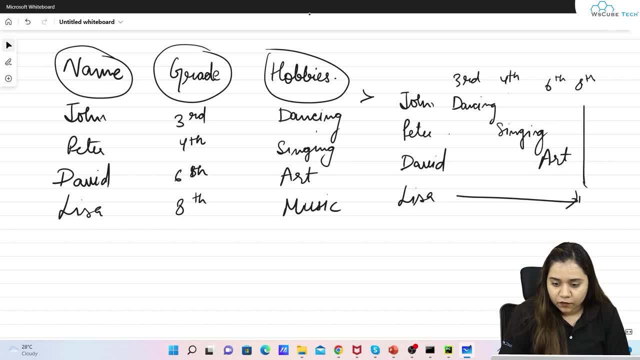 lastly, on Lisa and eighth: over here we will have music. So now we will get the output and the values, the empty values over here. these will be what These will be, not a number values. that means these will be a nan values over here. 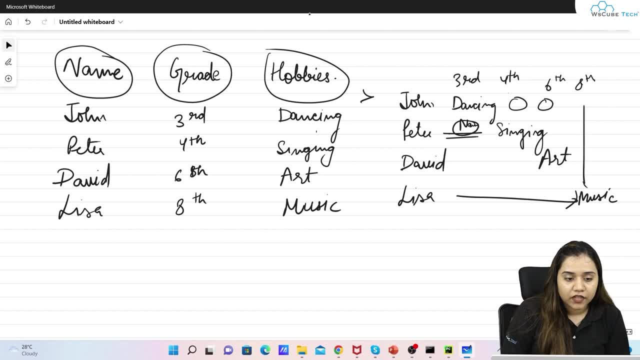 This is how we will get the output. Pivotting means that we will pivot the values in such a way that it will take 3 parameters. the first one would be for the rows, the second one would be for the columns and the third would be the data. So here we need three columns. 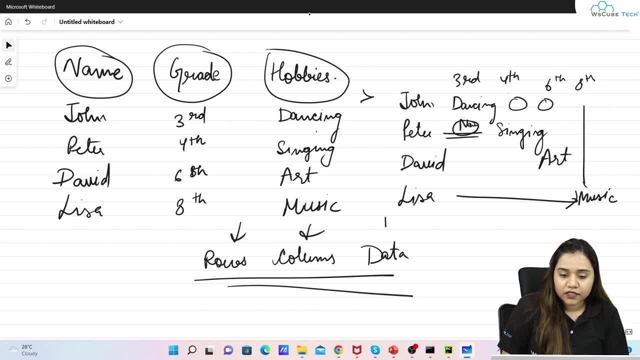 basically, one will get converted into rows and second one will get converted into columns and the third one will be converted into data. over here We can give multiple data as well, If you want. you can. if you want, to give it another data frame with another column, if裹 preventable withheit рокup to a large number of data frames. So you want to create another data frame with. 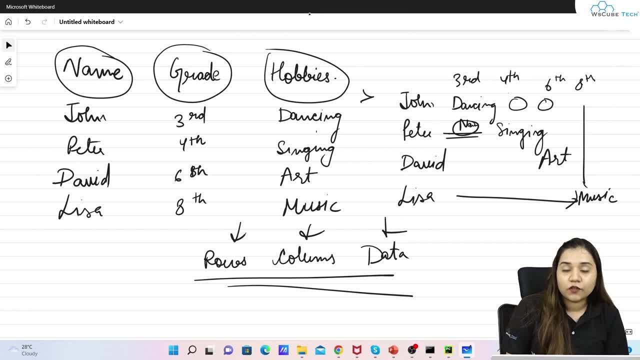 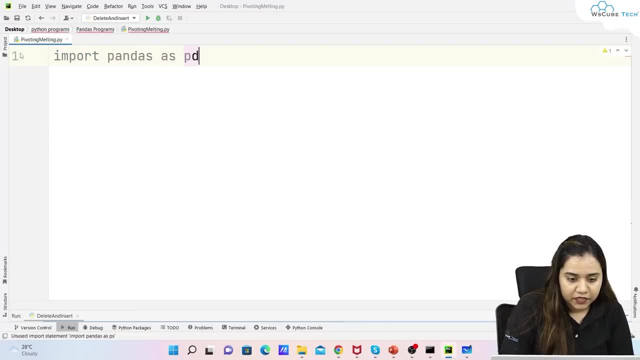 other data. you can give multiple data as well. over here, let's have a look on how p voting works with the help of pyjama. so first of all, i will import pandas over here. so import pandas as pd. once we have imported pandas, let's create a dictionary over here. so i'll be creating a dictionary in. 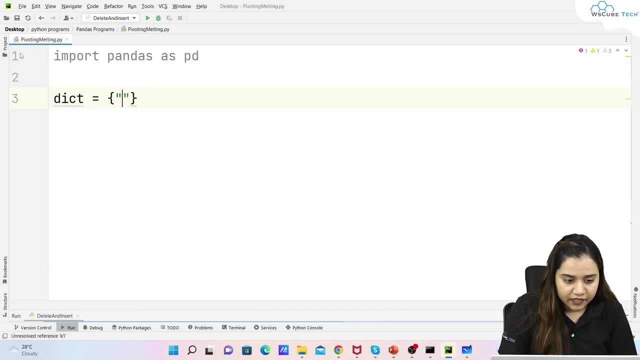 which we will be having. let's say: first one is k1. i'll be creating a keys over here, so i'll be just creating keys. keys would be in the column. i will be passing a list that will have k1 comma, k2 comma, k3 comma, k4 comma. we'll be having another values that let's say so after keys. we have, let's say, the. 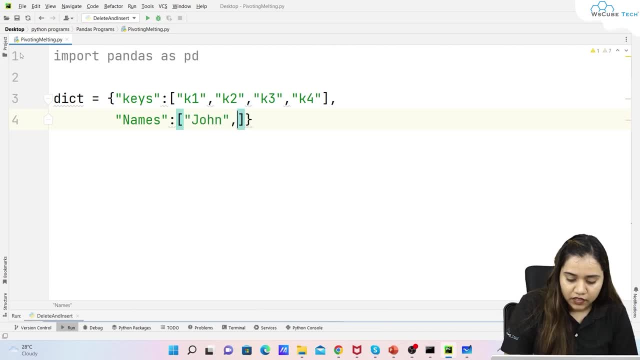 names, the names of the student. so we have john, then we have lisa, then we have david and lastly we have peter. after this we will be having their hobbies or we can have their houses as well. so, if you know so, just like in schools, we have different houses, like if someone is in red house, green house, 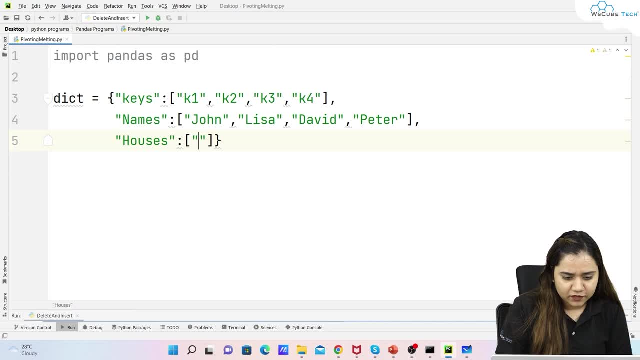 blue house, yellow house. not you yellow, but gold. we say generally. so we can keep those houses over here. so let's say that someone is in red house, we'll give red over here, then we will give blue. the other one is in blue, then someone is in a, let's say, green, and one more. 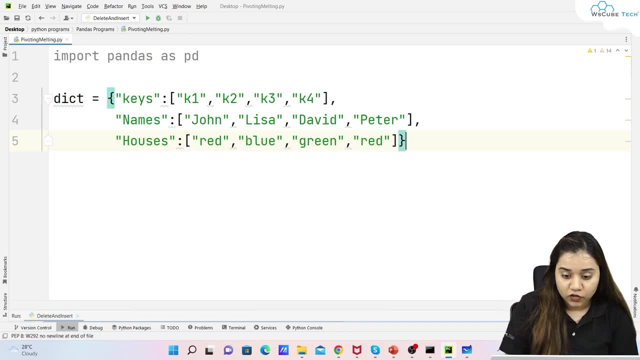 over here is in red because majority of students- i don't know- somehow goes in a red house. okay, so this is how we have houses over here. now, what we need to do: we need to apply the method of pivoting over here. to to apply that, first of all, let's create a data frame. the df is equals to pd. 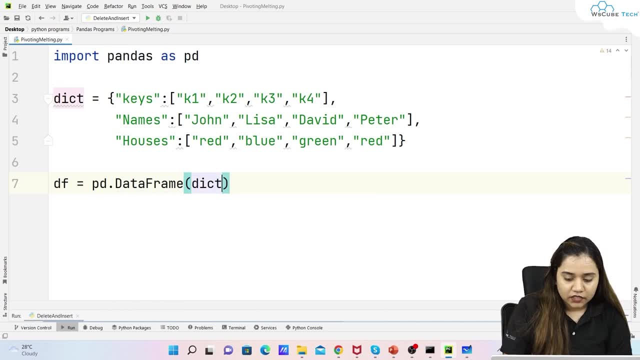 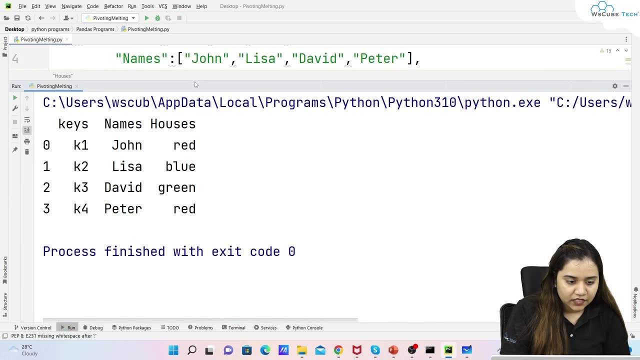 dot data frame and here i'll be passing our dictionary and let's run it as a pdf, and we'll be running it as well by printing df. as soon as we run it, the output that we will get over here would look like this: that we have one column, that is keys. the second column over here is names. then 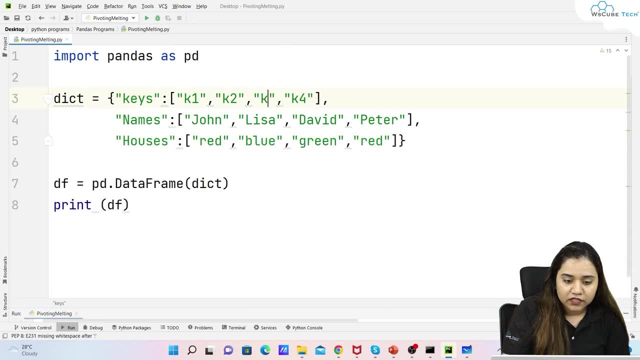 we have houses for keys. let's keep them as k1 and k2 over here, that these keys are k1 and this one is k2, so we will have only two types of keys over here: k1, k2, k1, k2- so that the data will get. 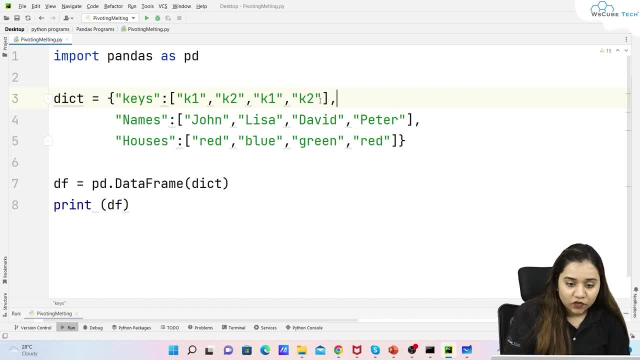 distributed in the two column and the two rows only. so this one will get converted into rows, this one will get the names will get converted into the columns and the houses will get converted into the data over here. so here i'll be writing: print df, dot pivot. inside the pivot we'll 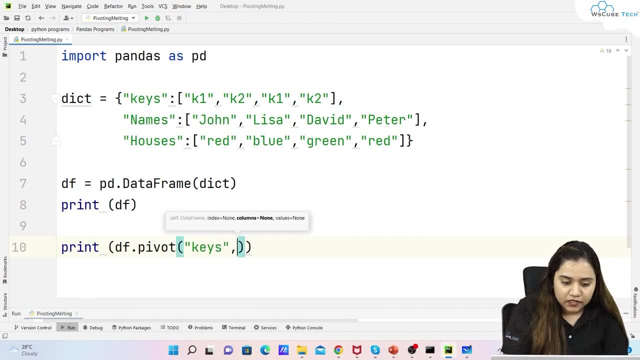 be passing three parameters. the first parameters will be the rows, that is the key. the second parameter would be the names, that is, the columns. and the third parameter would be the data, that is, the houses. and as soon as we run it, let's have a look on what output we'll get over here. so this: 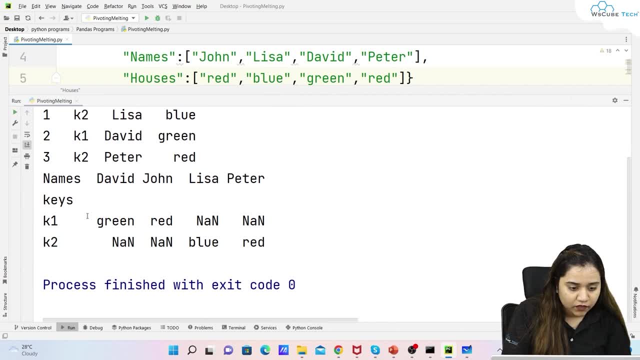 is how we'll get the output. you can see that we have in the k1 we have green and red, because here we have green and over here we will get blue and red in peter and lisa. this is how we have obtained the data that in the the rows, the rows over here are k1 and k2. the columns over here are names that 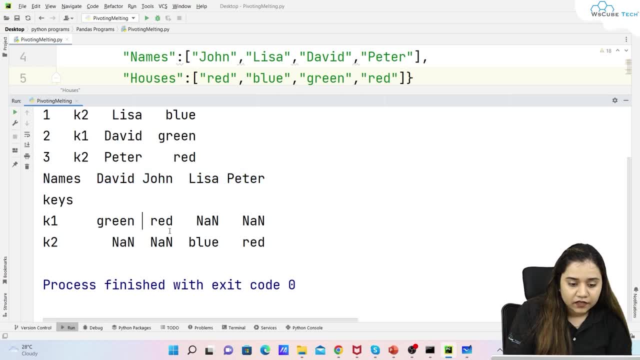 is david, john, lisa and peter and the data over here is green, red, blue and green. that has been distributed inside the rows and columns. the empty values over here are nan values. this is how we have obtained the data. suppose if there was more data, there were, let's say, grades over here as well. 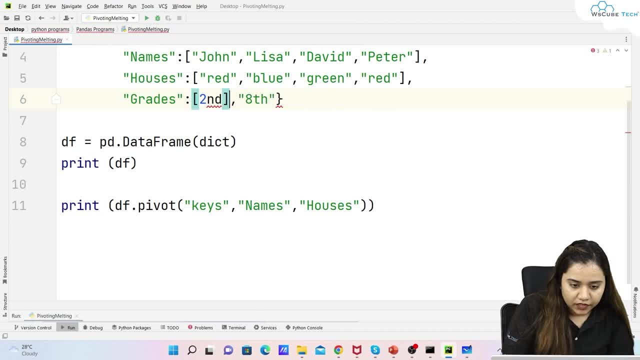 someone is in second grade, someone is in eighth grade. what I have done, let me just write it again. so someone is in, let's say, second grade, someone has, someone is in eighth grade, someone is in ninth grade and someone is again in third grade. in that case, um what we will do, the house is the part of. 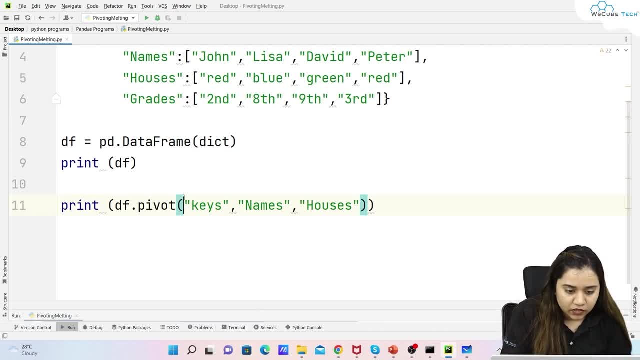 the houses will become what in that case? what would happen? this one, uh, I'll just write it in this way that over here, index will be the keys, comma columns will be the names and the values would be the houses. and here we can pass a dictionary. sorry, 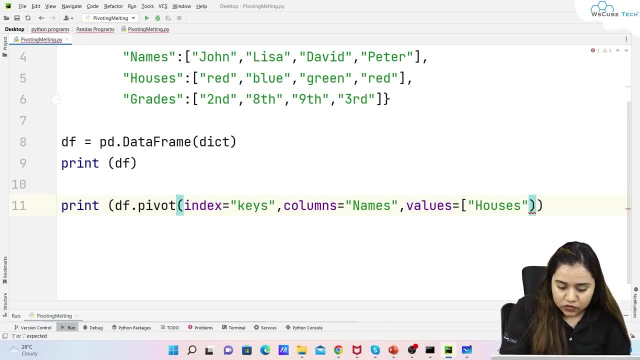 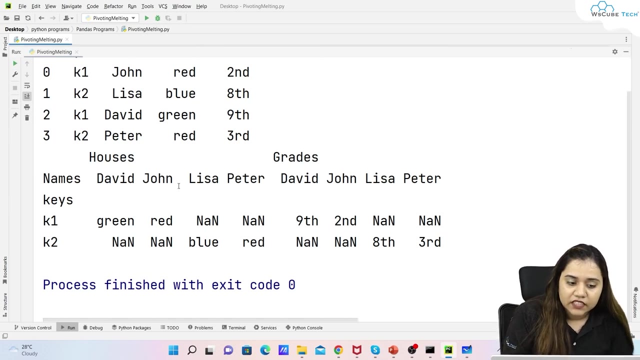 a list over here that we can write a list that has houses and grades. so I will write grades as well inside the double quotation and let's close the list also over here now. if I run it, the output that I'll be obtaining over here is that I'll be obtaining two data frames basically inside the one. 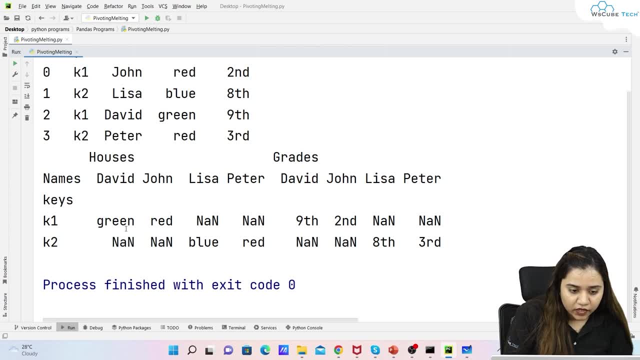 which which has columns as names, the rows as K1 and K2 and the data over here inside it, as this one has houses and this one has grade over here. so this is how we will be obtaining the output, so you can- you can pass multiple values also over here and the columns obviously will. 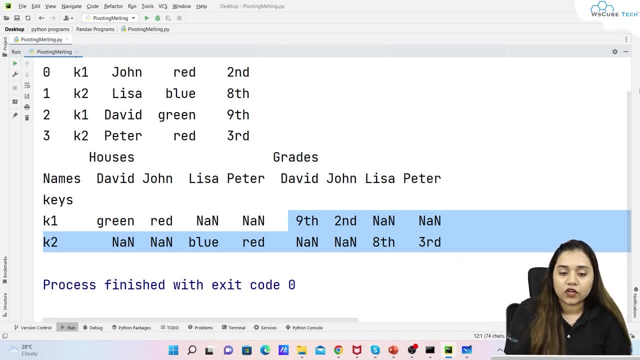 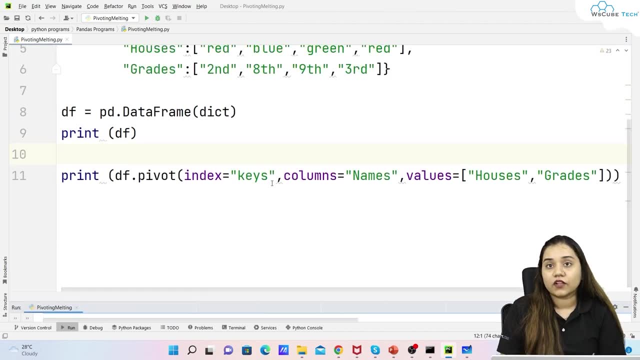 remain one. you cannot create multiple types of columns, but you can create: the columns over here will remain one and the rows over here will remain one. that means you can pass one value over here. okay, this is how our concept of pivoting works. now let's talk about what is melting here: the 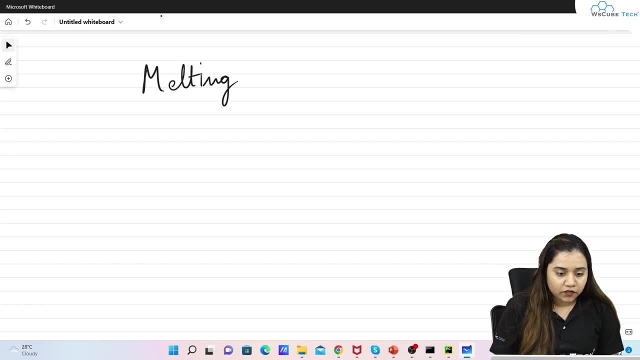 concept of melting over here says that suppose, if you have three rows, uh, three columns. basically let's say you have names, then you have grade and then you have houses. okay, so names is let's say: first we have john, then we have david, then we have peter and lastly we have lisa. similarly in the 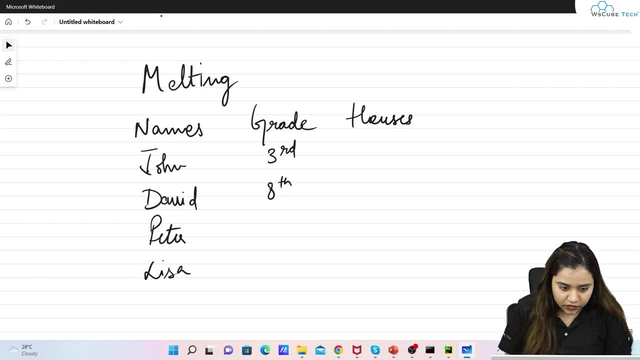 grade. we have third, we have eight, we have nine and we have tenth. in the houses we have red, blue, green and blue again. okay, so you can see that the concept of melting over here says that suppose, if you have three rows melting over here, says that here one whole column will become what a whole column will become the. 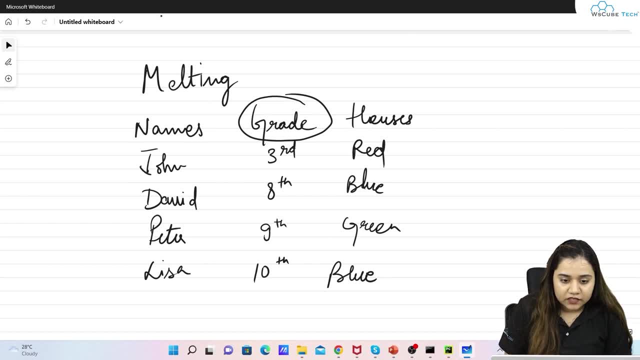 values of a whole column. that means here it will get converted in this thing. the name of the column will get converted into a variable and the value inside it- that means a third, eighth, ninth and tenth- will get converted into the values. the new one would look like in this way. that suppose we. 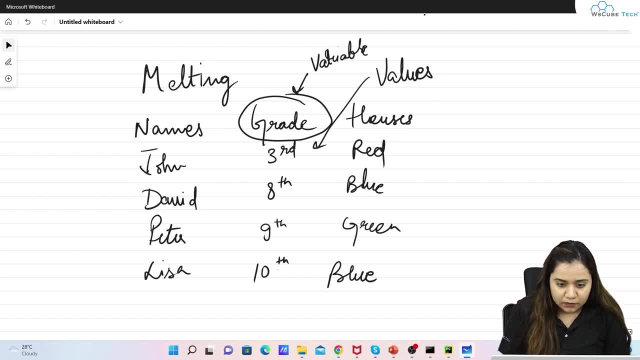 have names similarly. just, we'll just ignore the names right now, so the names will come over here, just like this, but here in front of it what we'll get? we'll get variable as a third variable as grade, grade, grade. it's actually grade and again grade and the value inside it that 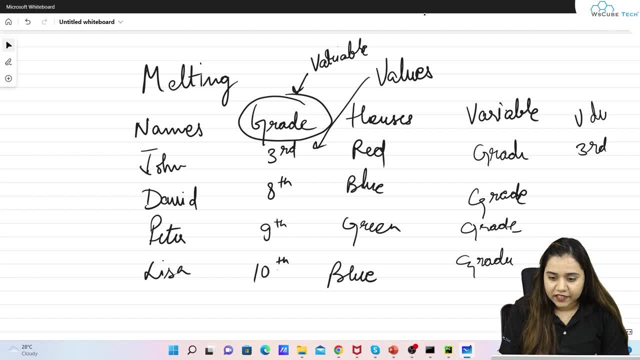 means the value would be third. so another new column will get created. that would be the value. so value over here would be third, eighth, ninth and tenth. that means this whole column will get melted in the form of two more columns. that means one of the, the name of the column will get. 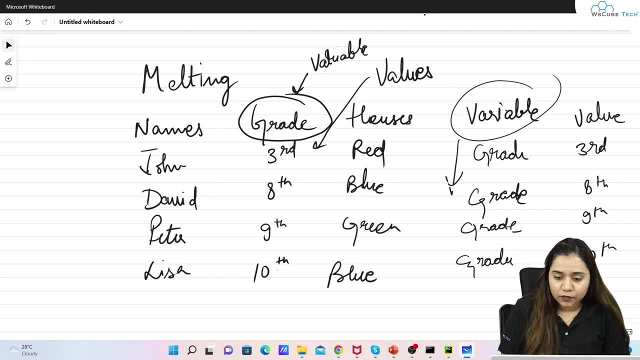 converted into a variable and its value. inside it would be the grade, grade, grade, and then the value is over. here that means whatever data is there inside this column will get converted into a new column which will be called as value, and the new values will get and the values which are there. 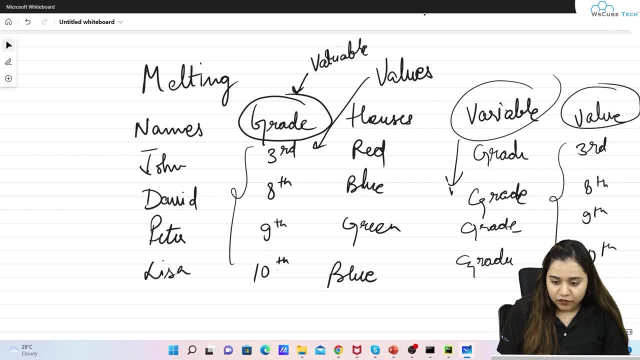 that means all the data which is there will get it converted in the format of this. okay, this is how like we will get that. the grade over here is third grade over here is eight, grade over here is nine, grade over here is ten. similarly, if you want to add houses, also over here you can add houses. so 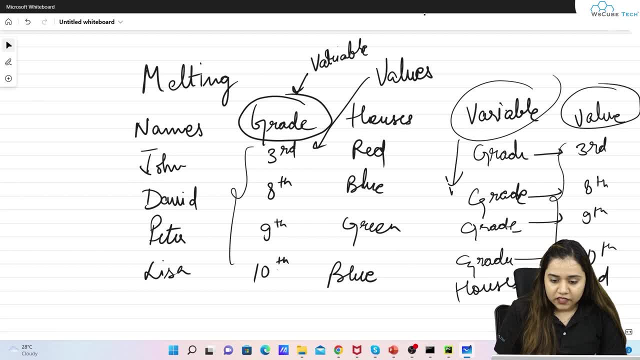 houses over here is red and then houses next house over here is blue. so it will keep going on in this way that this will get melted. one column will get melted and create a two separate new columns, which in which the name of the column would be a variable and the values inside it, that means, the data which. 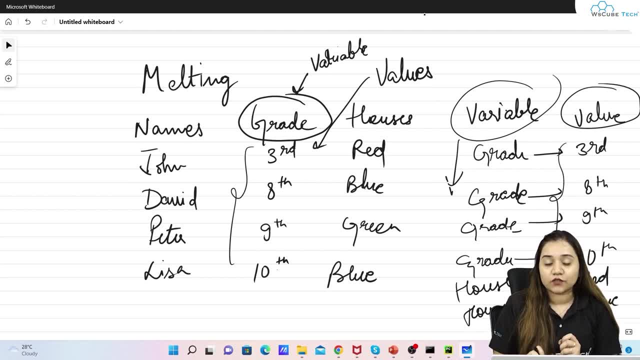 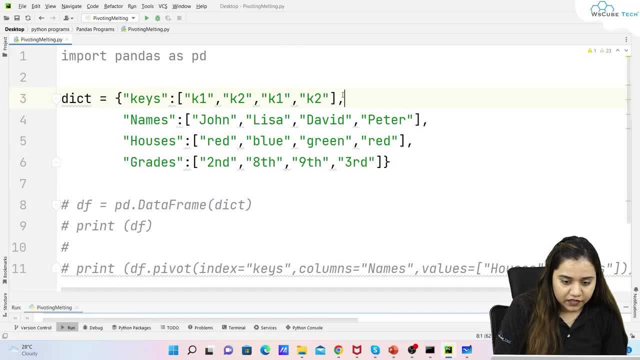 is there inside. it will get converted into a new column that will be called as values here. okay, let's have a look on how this can be obtained in our pie chart. so i'll just put this data inside the comment and here from here i'll remove this keys part. okay, so we have this as our dictionary. 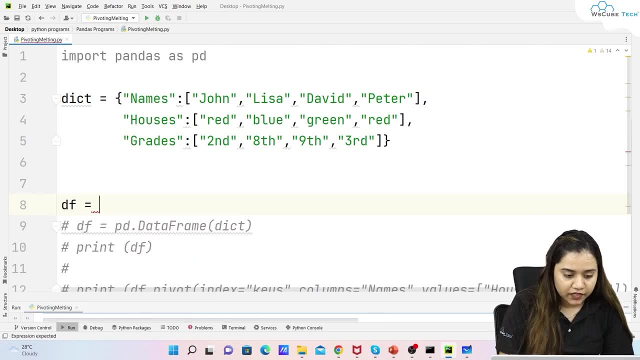 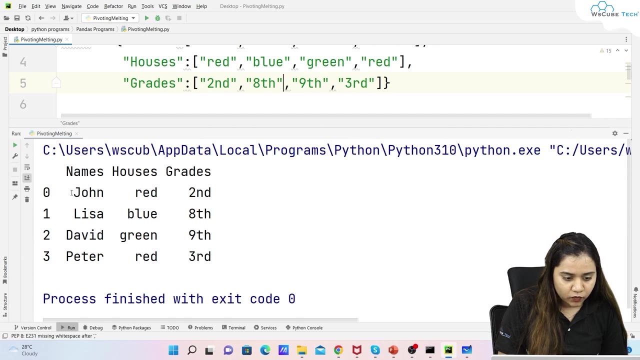 how to melt a data frame. first of all, let's create a data frame. so for that we will be writing df is pd dot data frame. here we will be writing dict and we will print df. let's run and see what output we'll get here. so as soon as we run it, this is the output that we are getting over here: zero one to. 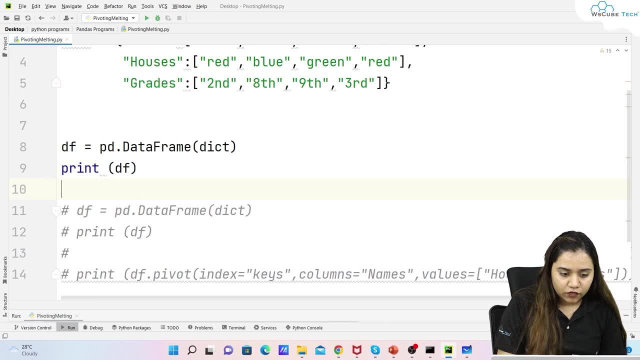 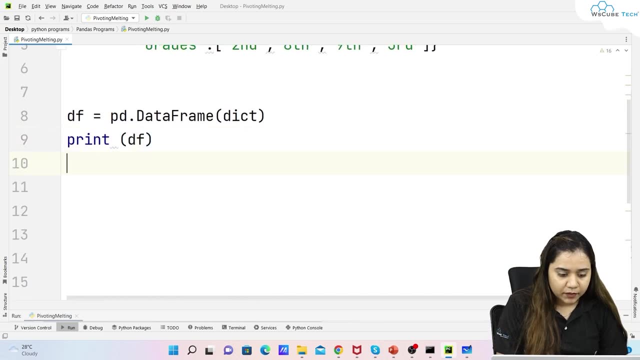 three: name, houses and grade. these are the three columns that we are obtaining now if we want to melt it. for melting it, what we will be doing, we will be writing here- let me just increase the form size a bit. so for melting, we will be writing df, dot, melt. and what do we need to melt? we need to. 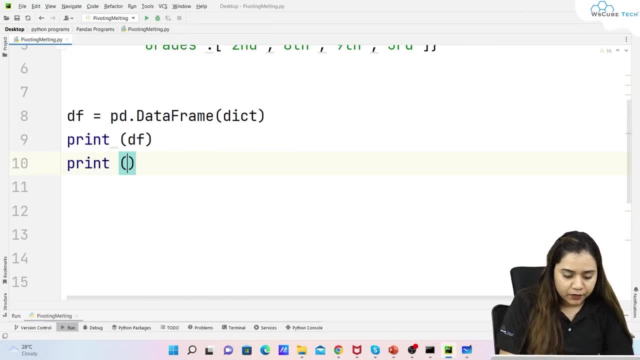 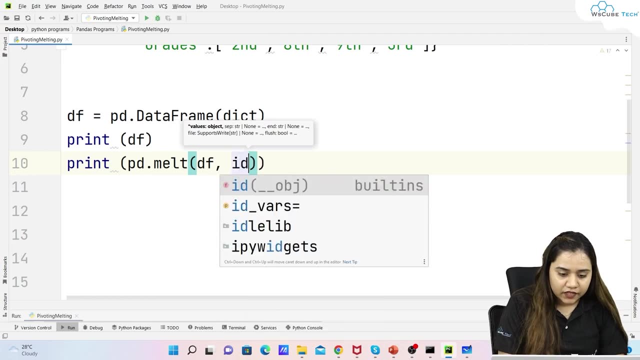 melt the data frame and to measure the data frame. what we'll be doing, we'll be writing pd dot. melt what we need to melt. we need to melt the data frame where the variable, the id variable would be, variable would be the names and, let's say, the value variables over here. 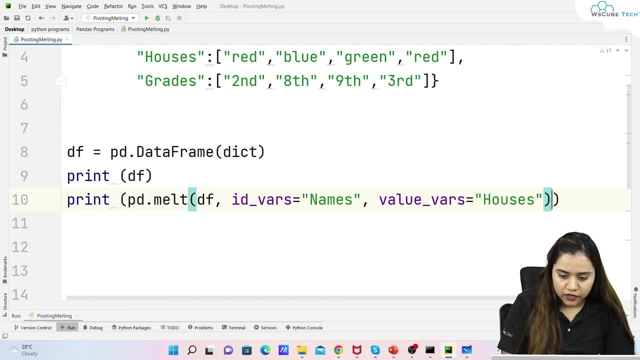 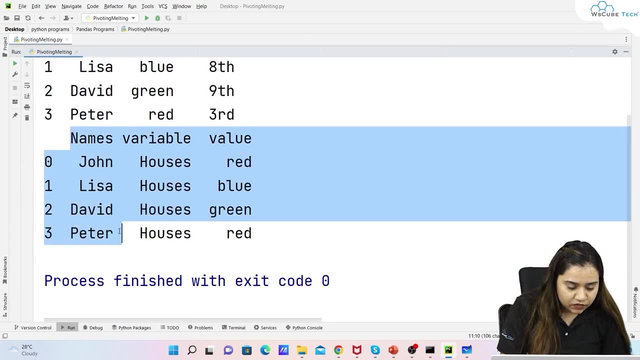 value variables would be our houses. okay, let's run and see what output we'll get over here as soon as i run it. the output basically looks like this: that we have names as the whole column, now next was id variable, that the next was value variables. that was houses over here. so what has 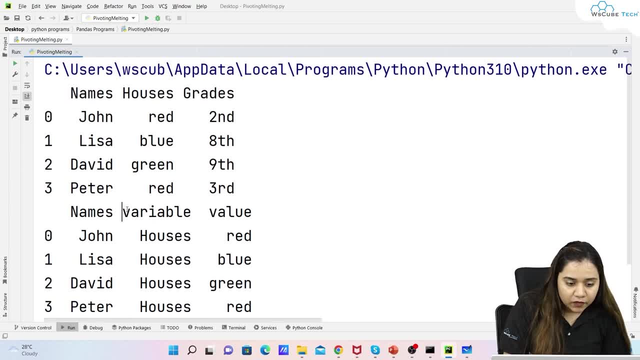 happened with the variable column, that means the houses column. a new variable column has been created in which all the values are houses and the values which was there in the house. that has been converted into another column over here which is called as value and inside the value is red, blue. 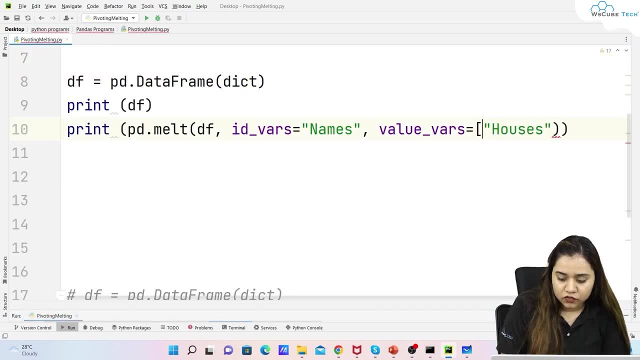 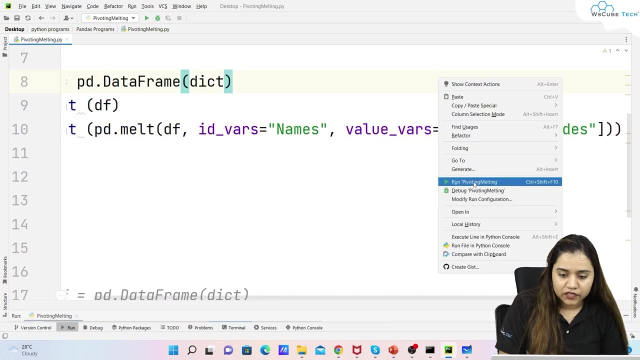 green and red again similarly, if you want to pass a list over here. so suppose in the value variables we want grades as well. so i'll be writing grades and let's enclose it, and now let's run it. so in that case, what will happen? in the variable section, only the grades will get added. so now we'll come. 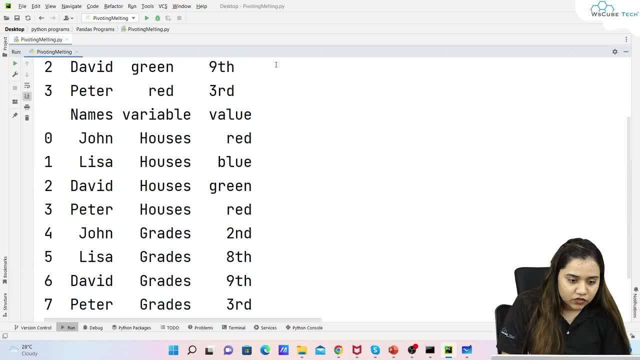 express 1 second nature case, which is known as points overall. in this case i'm ace and i'm replacing it with here, else it's not important thatอน inferior. Now in the variable we have grades as well, and their value has come over here in front of it. 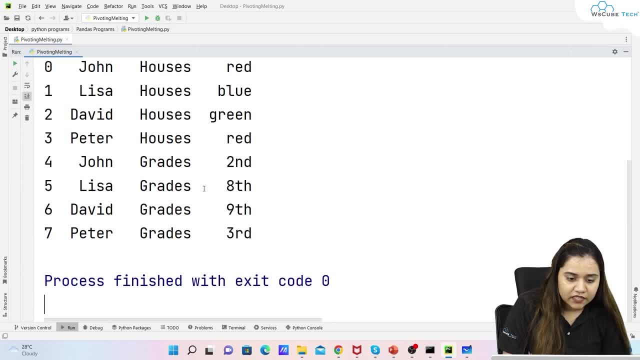 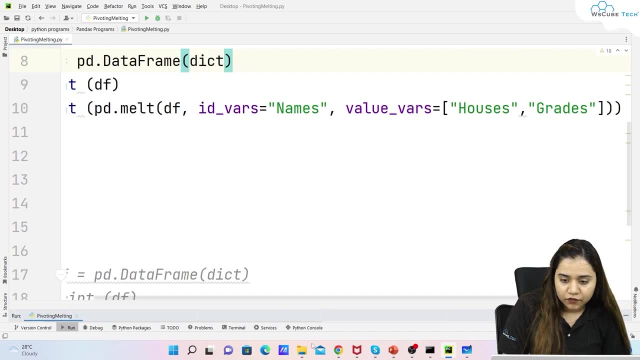 So the name also are repeating over here that John is in grade 2nd, Lisa is in grade 8th, David is in house green, Peter is in house red. This is how we have obtained the data over here: by melting the data frame.